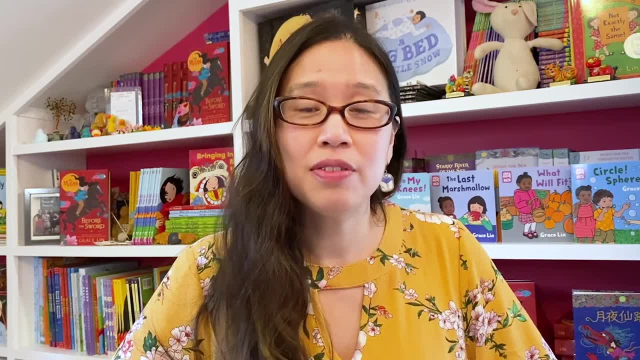 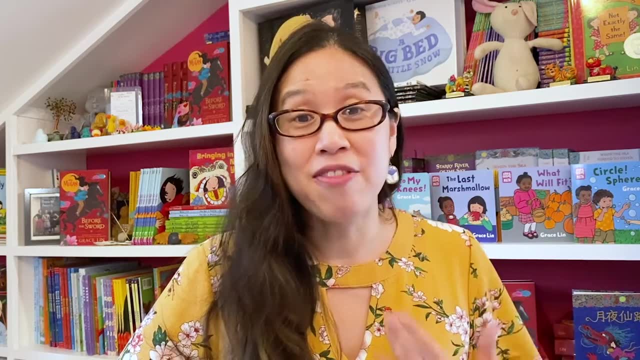 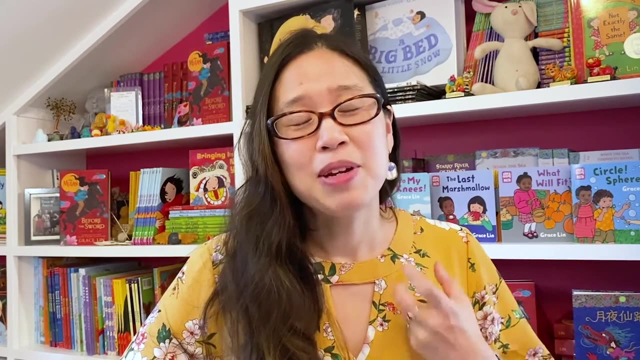 I would go to the bookstores and I would feel very frustrated Because I felt like I couldn't find any board books that reflected my family. I saw lots of board books with animals. I saw lots of board books with white characters, But I didn't see that many board. 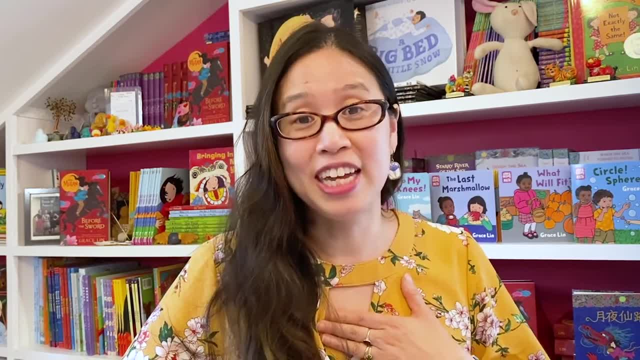 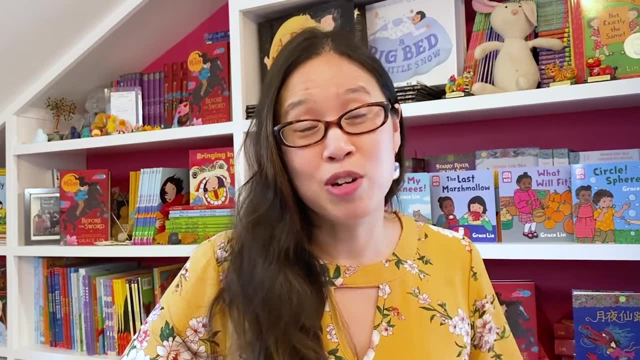 books that had people that looked like me and my daughter in it. So I was very, very eager to do a board book that showed more of the diversity in this world. We kept hoping and hoping we could come up with something that would work for us, And I was very, very eager to do a board book that. 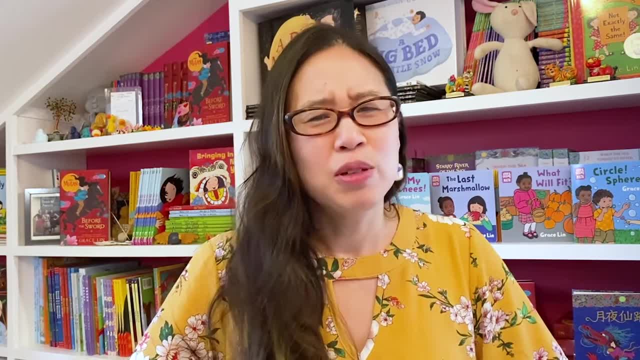 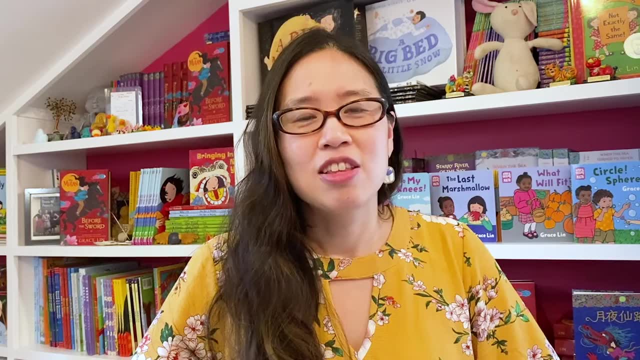 showed more of the diversity in this world. We kept hoping and hoping we could come up with something for a board book. And then one day she called me up and she said: would you like to do math board books? And I thought, um, you mean like numbers? And she said, no, it's more than numbers. And 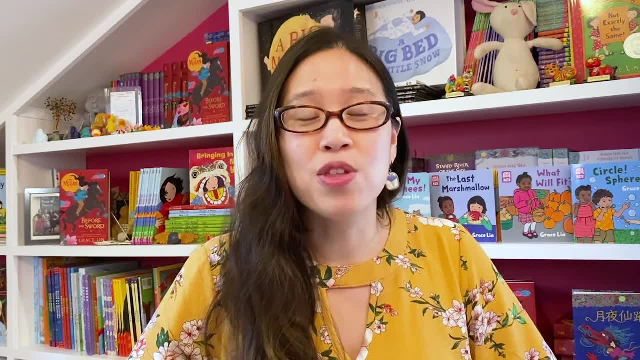 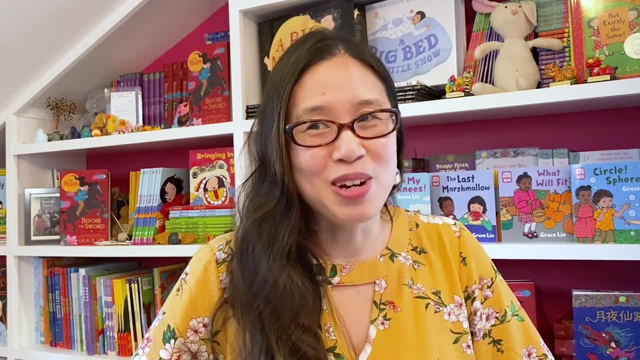 that's the whole point of this series: that math is more than numbers, that math is all around us, that it's actually commonplace and it's not something to be intimidated with, which is actually my very first reaction. when she came up to me and said math, I was like, oh, I'm kind of scared of math And she said, no, it's not. And I was like, oh, I'm kind of scared of math. And she said, no, it's not. And I was like, oh, I'm kind of scared of math. And she said, no, it's not. 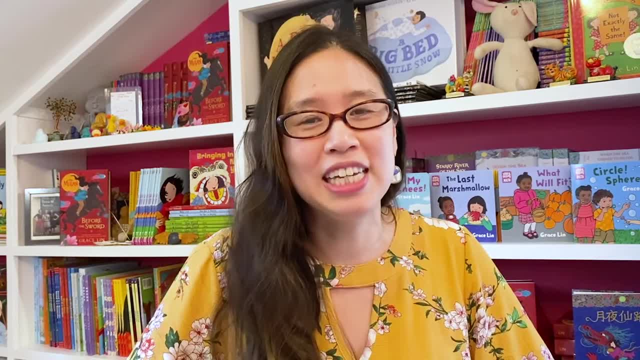 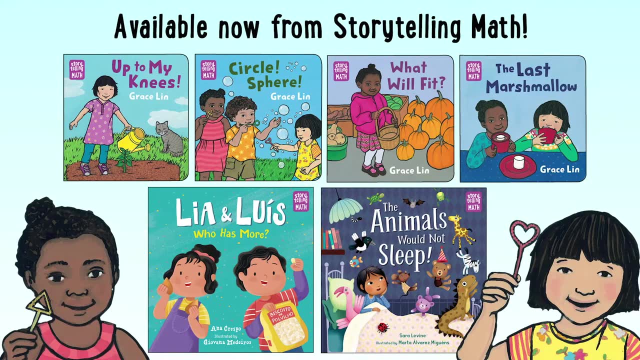 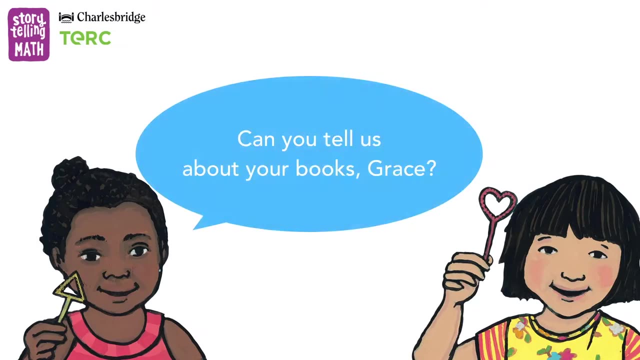 It's not something to be intimidated about, And that's what we want to teach kids and their parents. And now the first six storytelling math books are available. Look, Mae, it's us And our friend Manny. We do all sorts of fun things together. Can you tell us about your books? 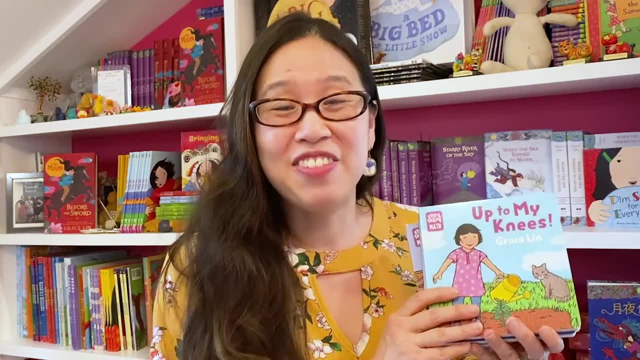 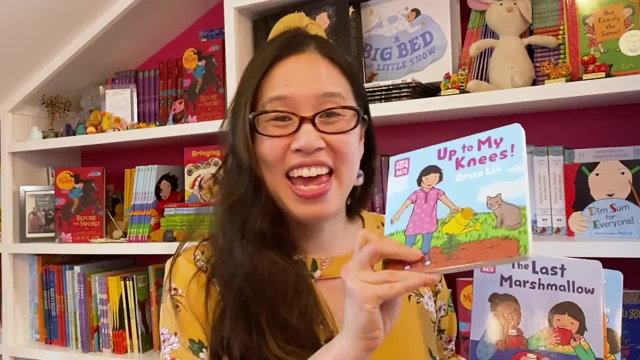 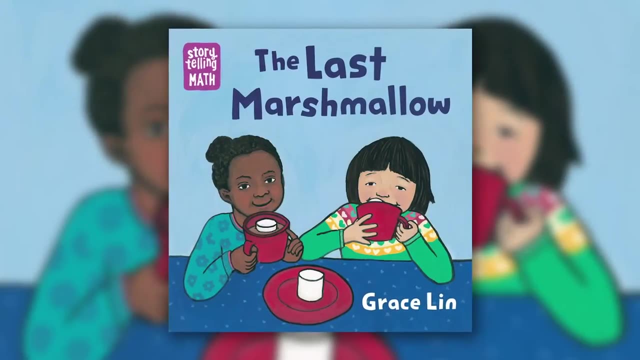 Grace. So these are my books and they feature three kids: Mae, who is the star of this one, up to my knees, And it's all about Mae growing a sunflower. It also includes Olivia, So this is a story about Mae and Olivia and how they have. 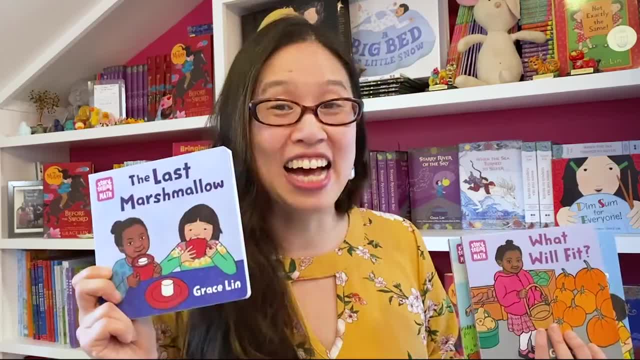 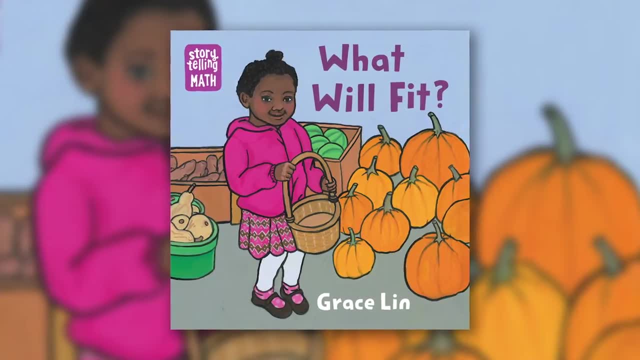 one marshmallow left between the two of them and how they have to figure out who gets the last marshmallow. And then we have this one that also features Olivia, which is called What Will Fit, And it's all about Olivia trying to find something that will perfectly fit inside of her basket. 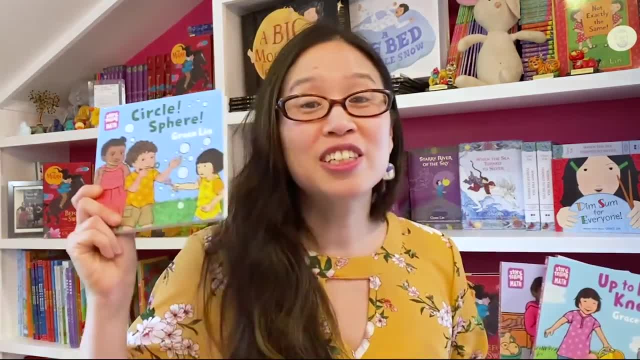 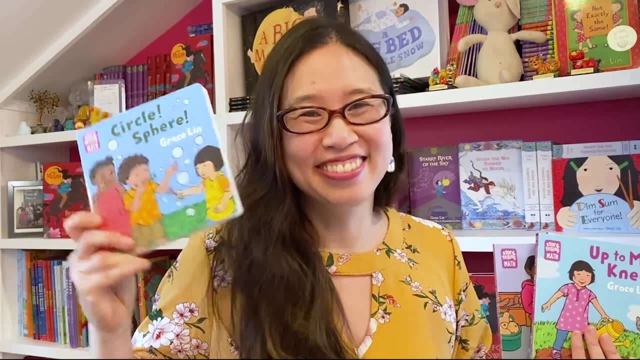 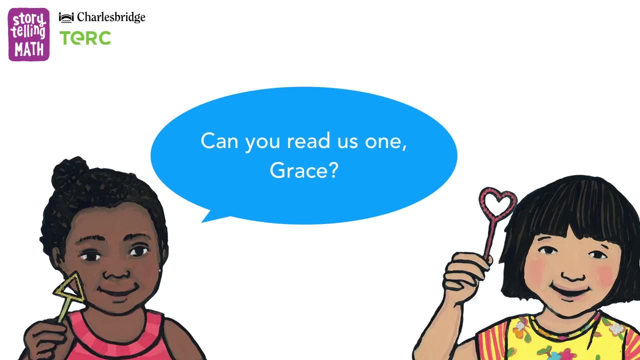 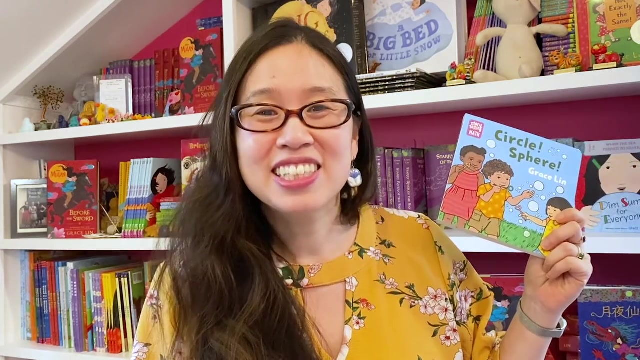 And lastly, there's this one called Circle Sphere, which features Manny, Olivia and Mae and how they blow bubbles. Wow, those sound like great stories. Can you read this one, Grace? Yes, I can. In fact, I read one of these books to some kids. I know I read this one, Circle Sphere. 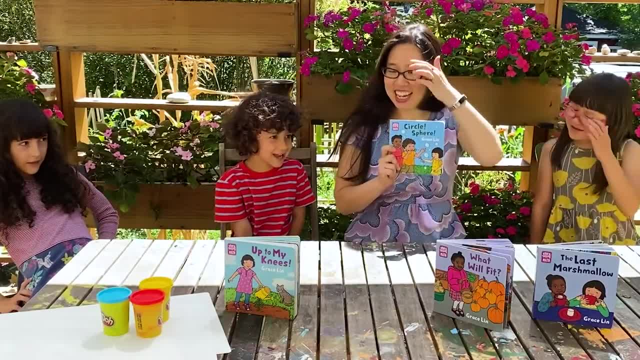 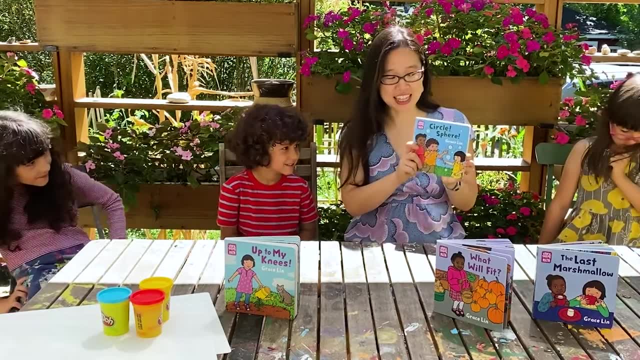 Let's take a look. You all know what a circle is, right? Yes, All right. But Hugo, do you know what a sphere is? No, You don't. Well, let's find out in this book: Circle Sphere. Now, this book is about kids blowing bubbles. 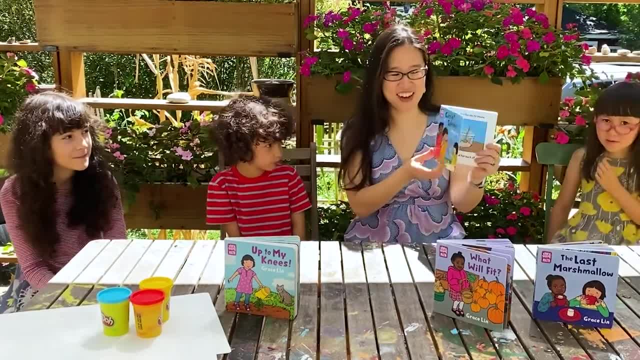 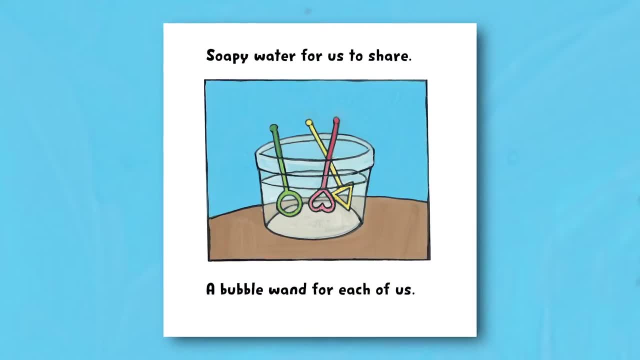 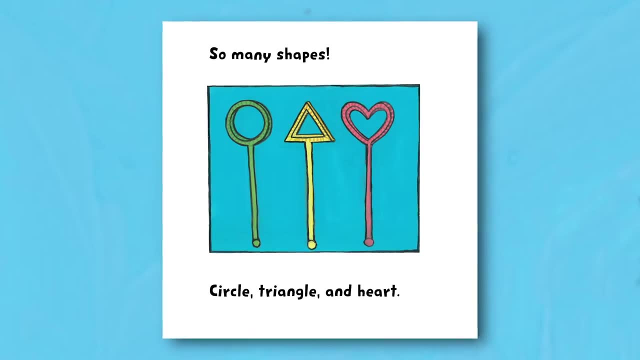 Have you guys blown bubbles before? Yes, All right, Let's see how they blow bubbles. Let's blow bubbles, Soapy water for us to share. A bubble wand for each of us. So many shapes: Circle, triangle and heart- See. so the bubble wands are all these different shapes. There's a circle. 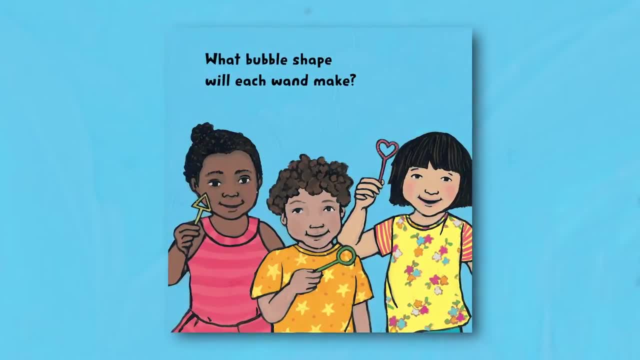 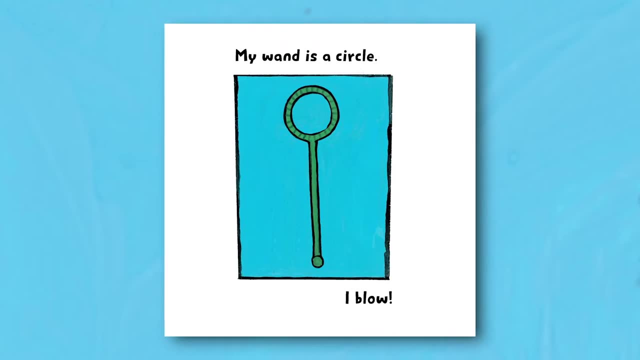 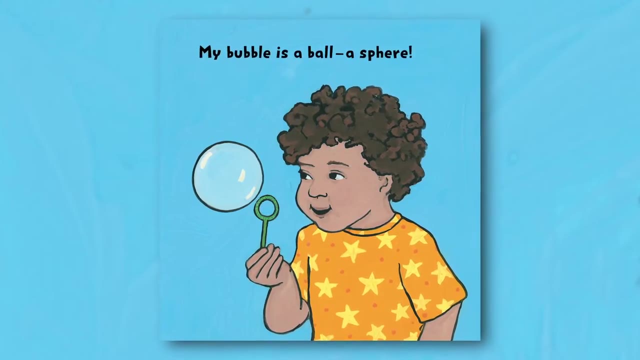 there's a triangle and there's a heart. What bubble shape will each wand make? My wand is a circle. I blow. My bubble is a ball, a sphere. So, Hugo, a ball is a sphere, Oh, okay. 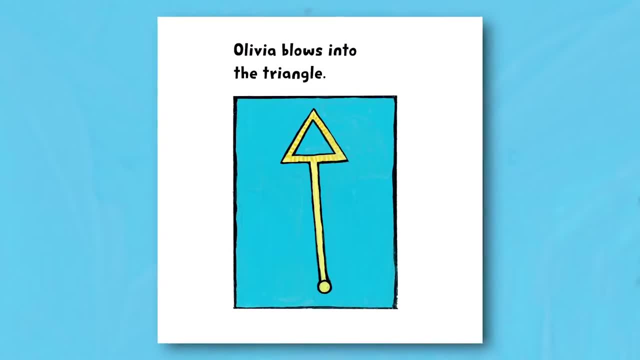 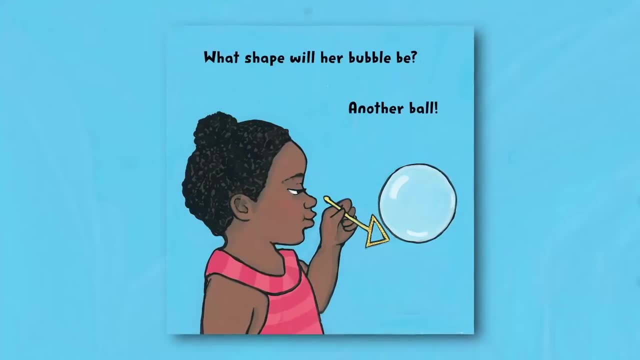 Olivia blows into the triangle. Do you think she's going to make a triangle bubble? No, A ball. I've never seen a bubble with a shape like a triangle- Me neither. What shape will her bubble be? Oh, it's another ball, So it's another ball. 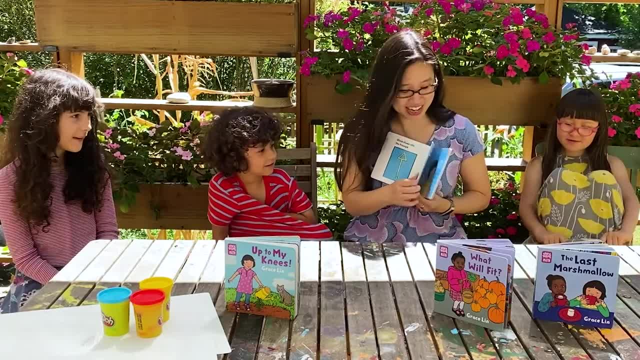 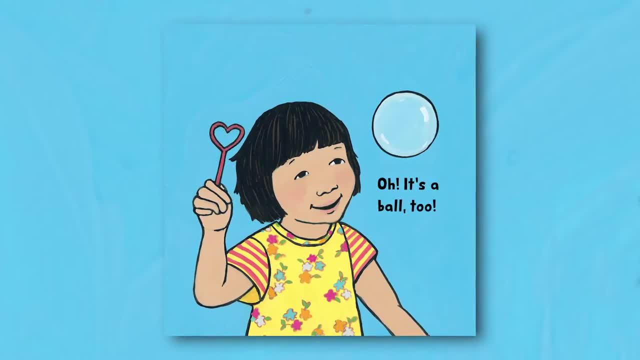 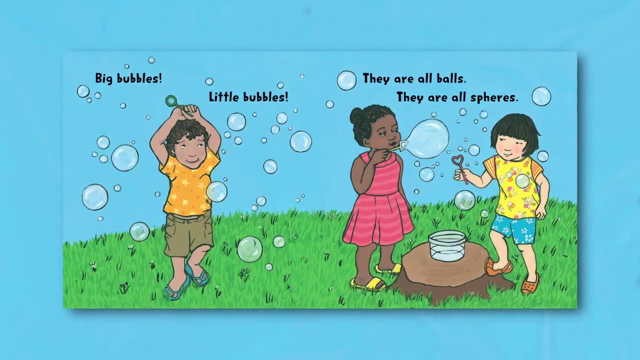 What kind? What is it, Hugo? A sphere, It's another sphere. Will Mae blow a different shape? Oh, it's a ball too. What's a ball? A sphere, A sphere. Big bubbles, little bubbles, They are all balls, They are all balls, They are all balls. 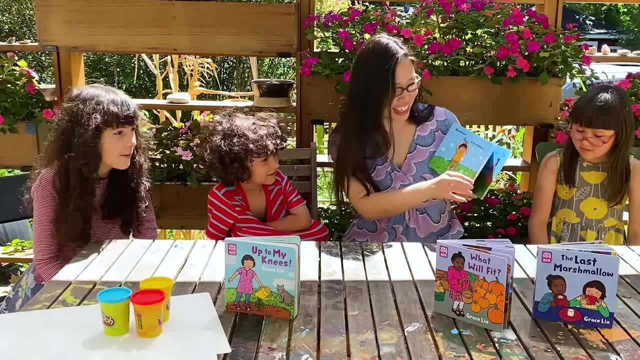 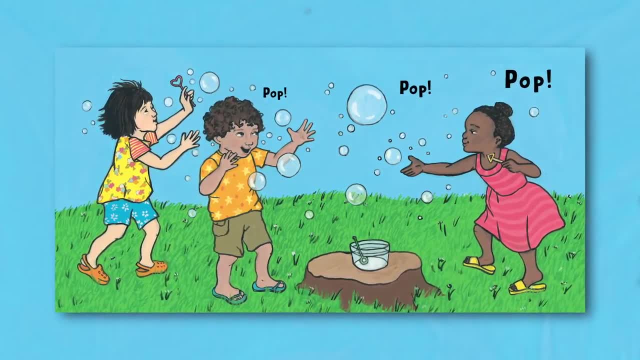 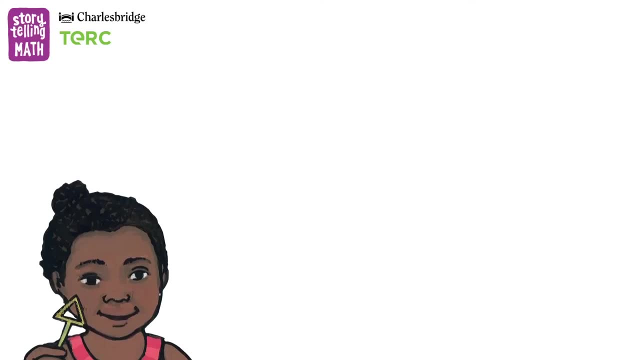 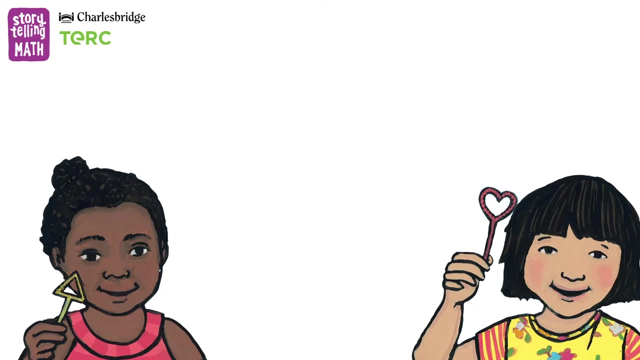 They are all spheres. Yes, they're all spheres. Pop, pop, pop, And they all pop too. So a circle is a flat shape, but a ball is a sphere. That was great, Thanks. I like that story, but where's the math? 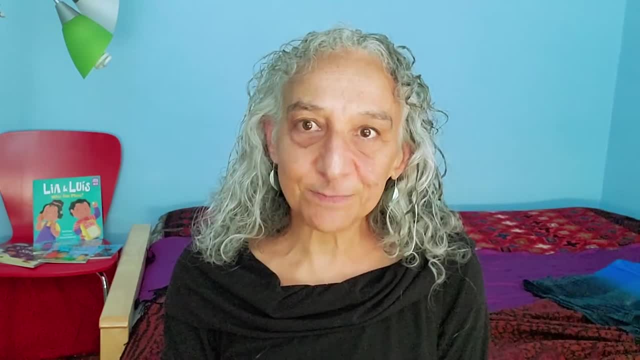 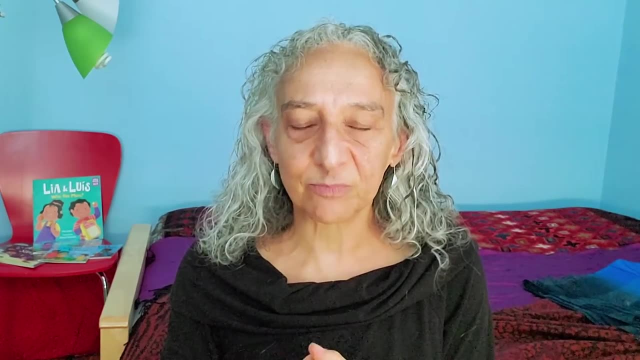 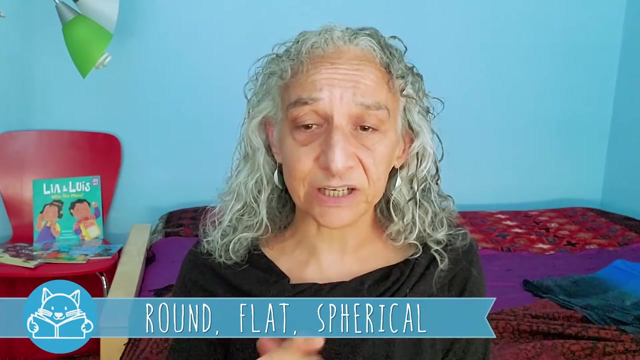 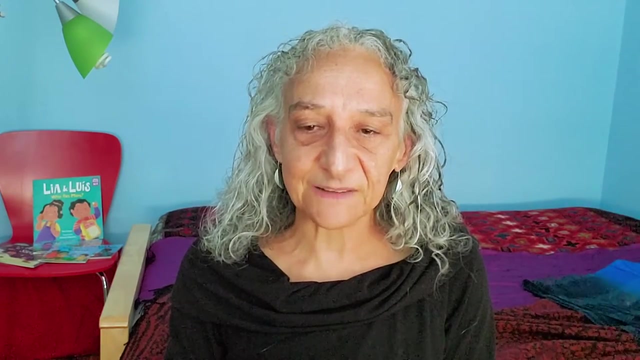 Young children learn about geometry by exploring the shapes of objects around them, Just like the children in the book do. This story takes the everyday experience of blowing bubbles and highlights the opportunities for children to engage with ideas like round, flat and spherical. And now Grace is going to show you one of our downloadable activities that gets kids investigating this math further in a very hands-on way. 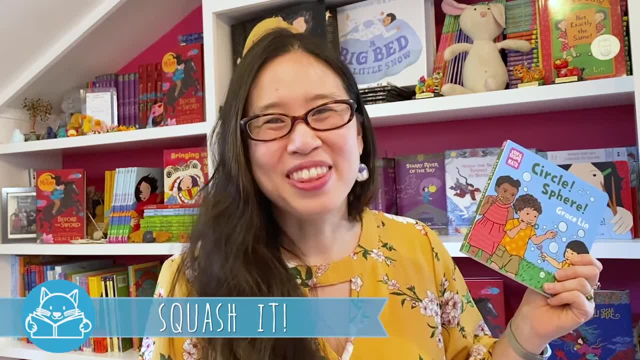 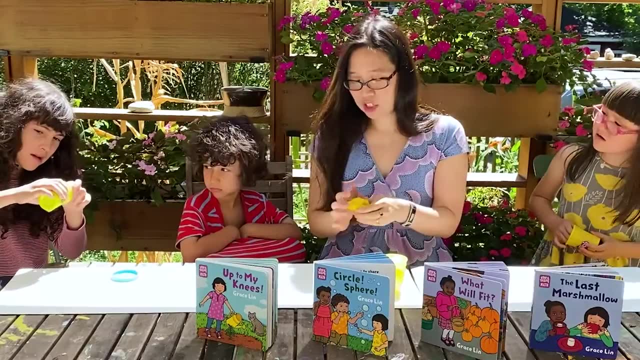 Yes, I did the activity squash it with the kids. I know Let's go take a look. What we're going to do now is play a really cool game. We're going to play a really fun game called squash it. So what you're going to do is you can make a shape out of your Play-Doh. 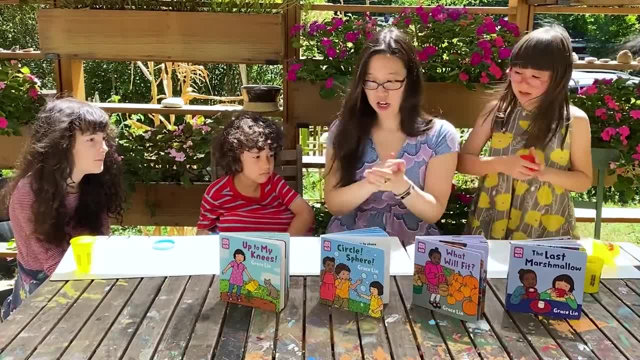 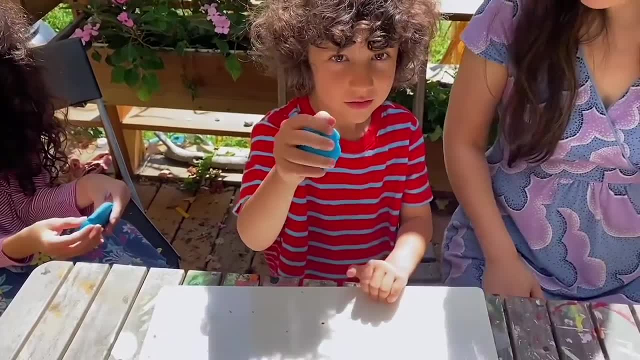 Make a shape. So let's see, I'm going to make a nice ball. You can make any shape you want. I made a sphere. Now squash it, Hugo. What shape do you think it will make when you squash it? 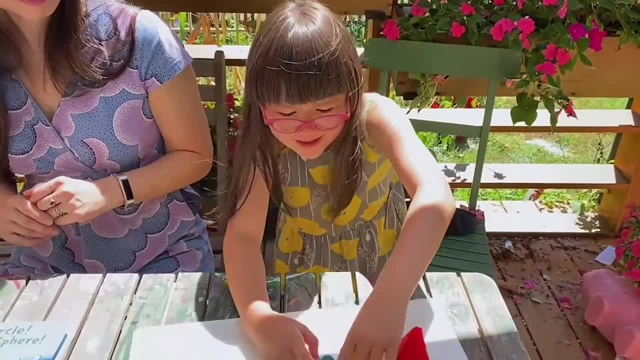 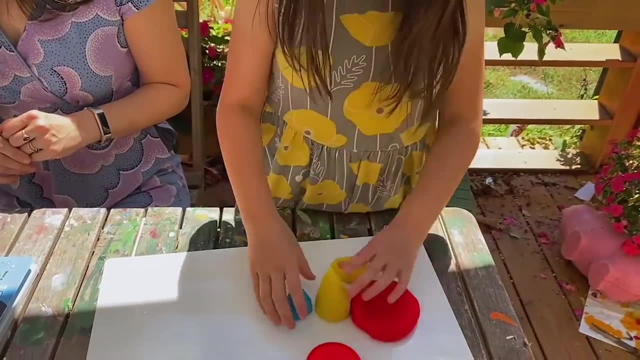 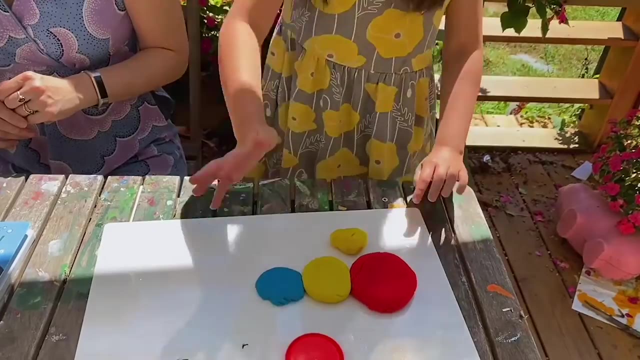 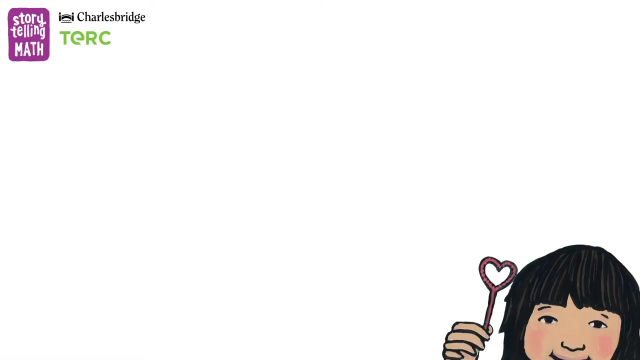 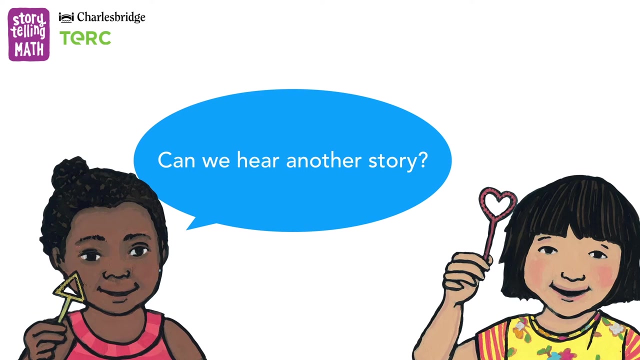 What did it make? A circle. I made three different cones, Wow, And each one made what shape? A circle. Yay, That looks like fun. I can't wait to try it. Can we hear another story? Sure, Olivia, Here's one of my favorites. 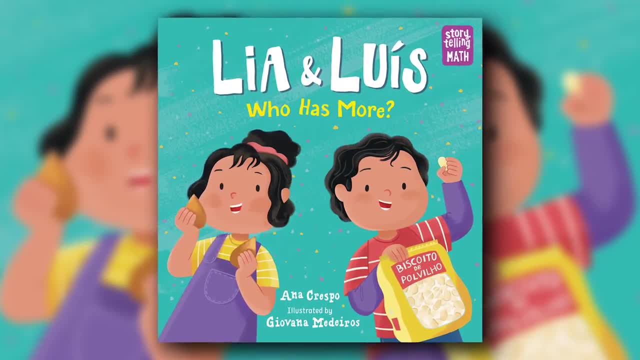 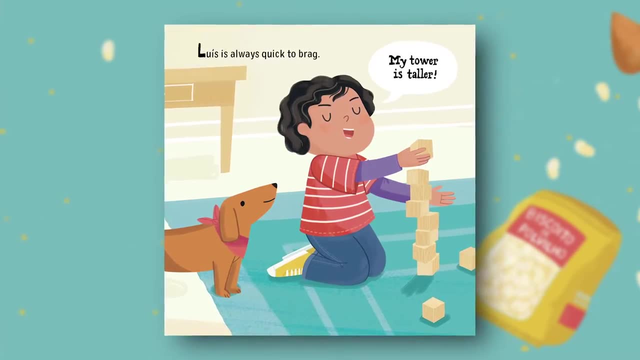 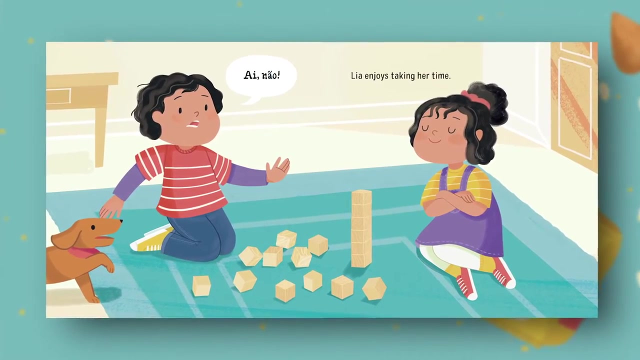 Leah and Luis by Ana Crespo and Giovanna Medeiros. I'll read the beginning of the story. Luis is always quick to brag. My tower is taller. Usually. his sister doesn't mind, I know Leah enjoys taking her time. 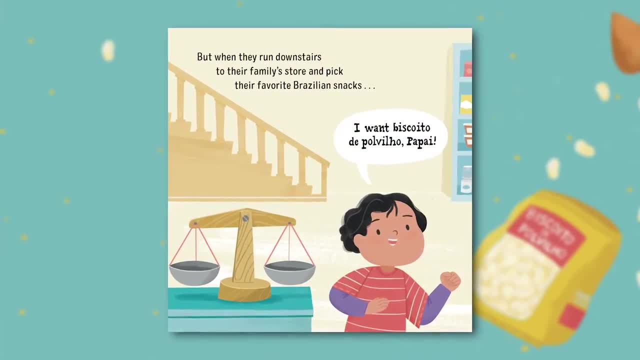 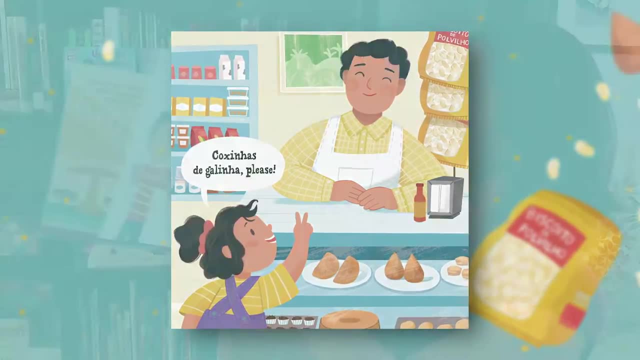 But when they run downstairs to their family's store and pick their favorite Brazilian snacks- I want Piscoito de Pavilho, Papai Casinas de Galina. please, Luis, starts bragging. I have more And Leah doesn't like it. 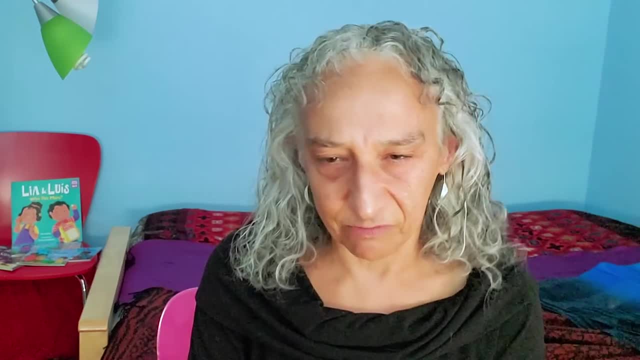 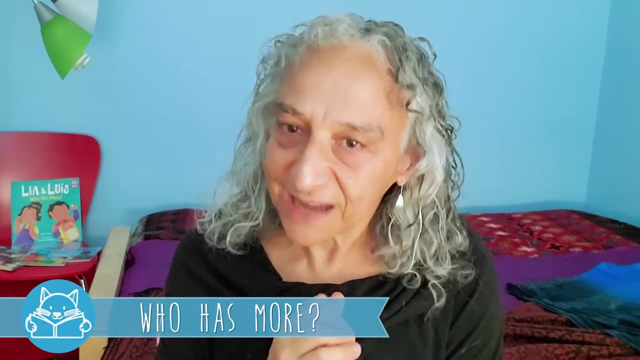 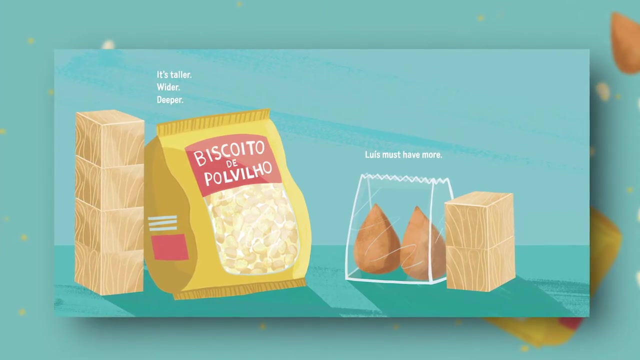 So it's a story about sibling rivalry. But where's the math? Well, they want to know who has more. Well, to find out, like all young children, they first look at size. Which one looks bigger? They find that size involves length, width and height. 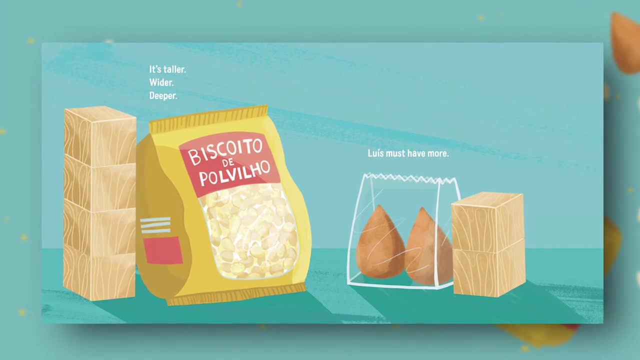 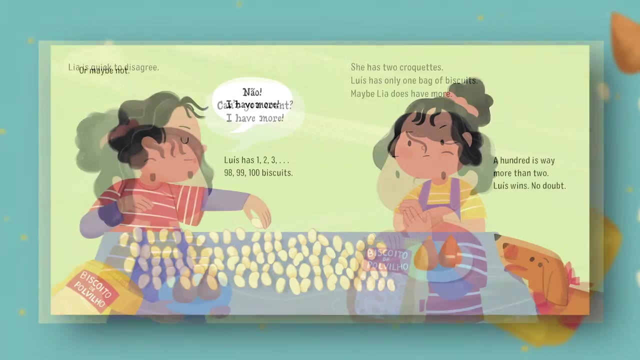 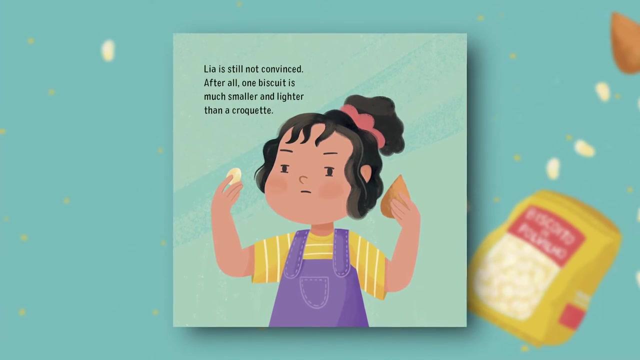 It looks like Luis has more. But next they consider amount. Leah has two croquettes, But Luis only has one bag. A hundred in the bag versus two croquettes. Hmm, then Leah realizes that one little Piscoito is smaller and lighter than a croquette. 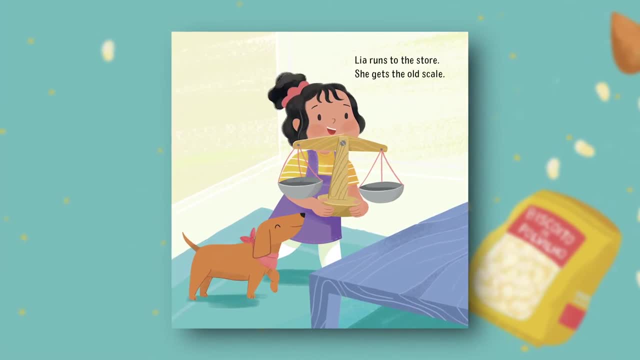 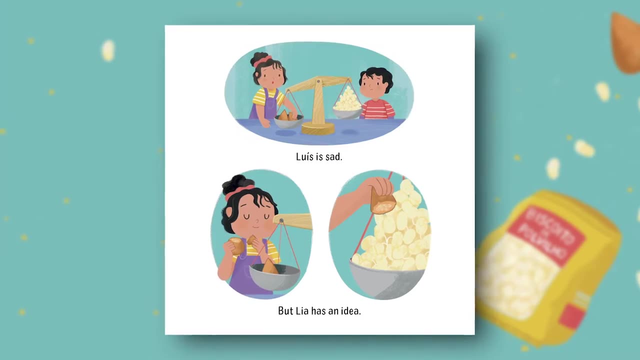 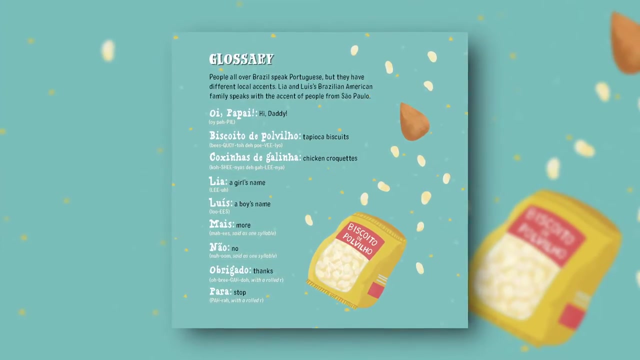 They decide to compare by weighing And Leah has more. Luis is sad. Can Leah find a way to make it fair so they both have the same? You'll have to read the book to find out. At the very end of the book is a Brazilian Portuguese glossary. more math, information and activity ideas. 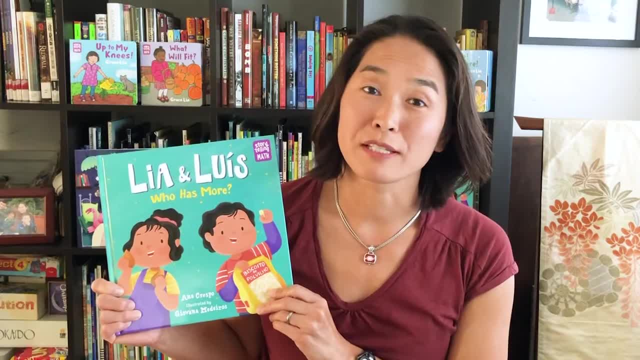 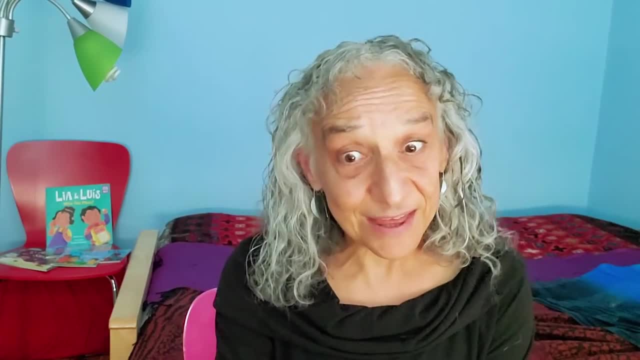 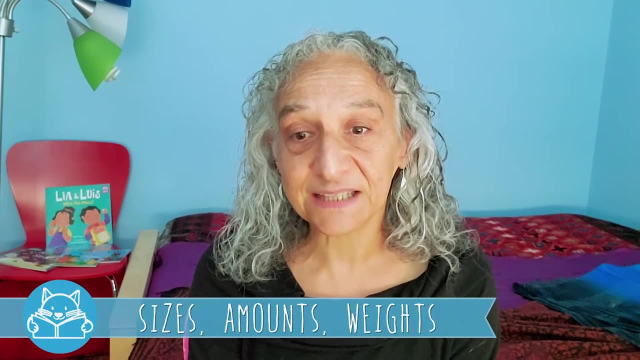 Both the author and illustrator of this story were born and raised in Brazil, So we have two own voices, creators who can bring their authentic experiences to the story. As for the math, Leah and Luis explore measurement the way young children learn best: By hands-on comparison of sizes, amounts and weights. 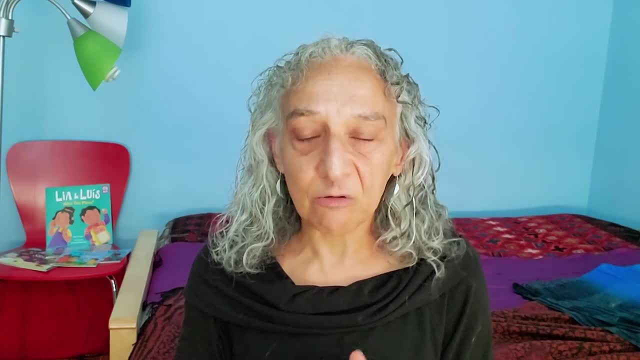 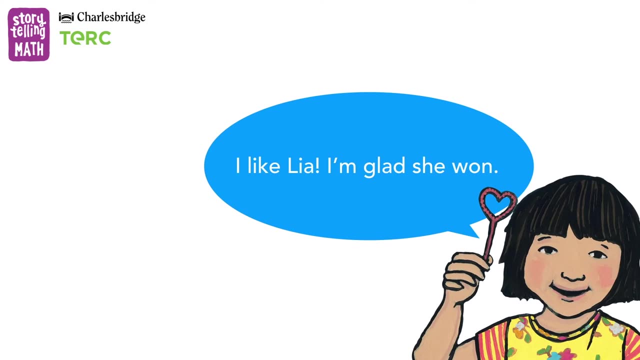 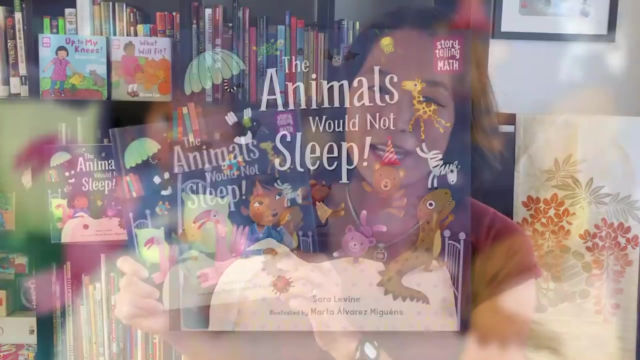 In this book, as in all of our picture books, readers get to see children's mathematical thinking in action. I like Leah. I'm glad she won Me too. What are the other stories about? In The Animals Would Not Sleep. it's bedtime for Marco and his stuffed animals. 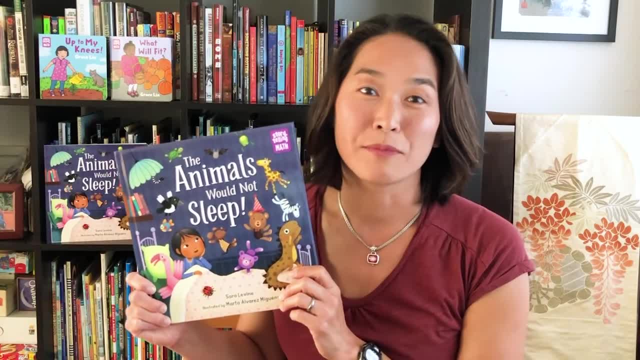 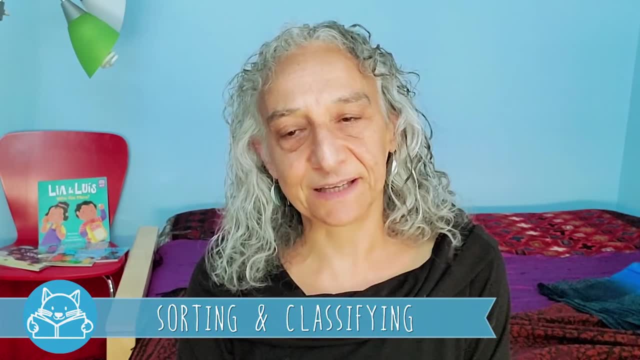 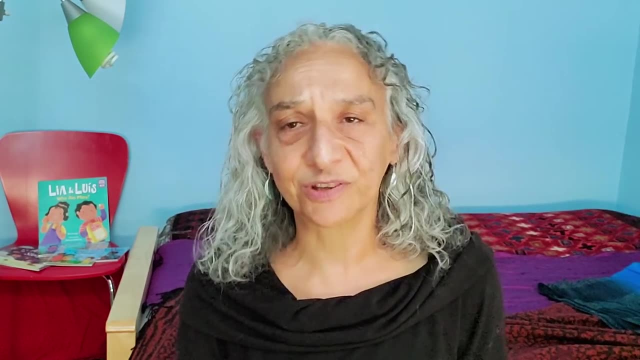 But the animals have other ideas. When Marco tries to put them away, they fly, swim and slither right out of their bins. This story involves the math of sorting and classifying. Marco combines mathematical thinking and empathy as he explores different ways to group the animals so that they're all happy. 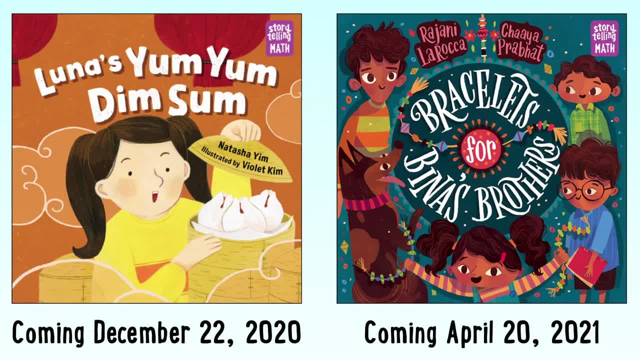 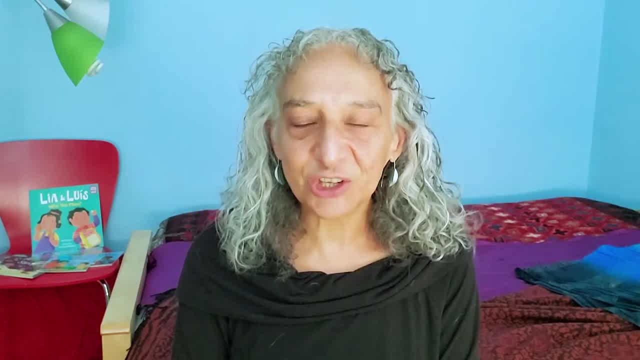 In Luna's Yum Yum Dim Sum. Luna and her two brothers have six fluffy pork buns to share, But then splat, Luna drops one. As the three children puzzle over how to share five buns, they grapple with division and fractions in a real-world context. 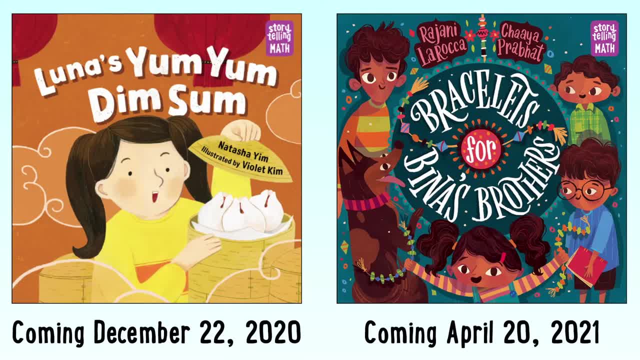 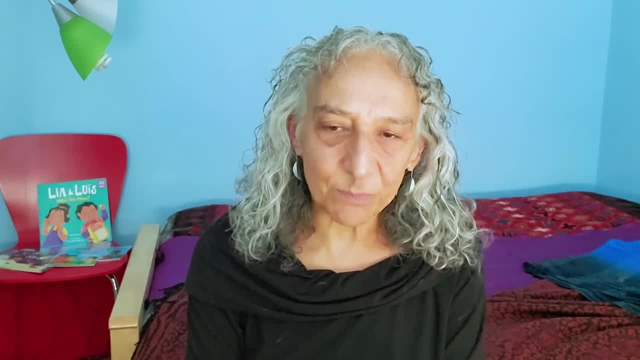 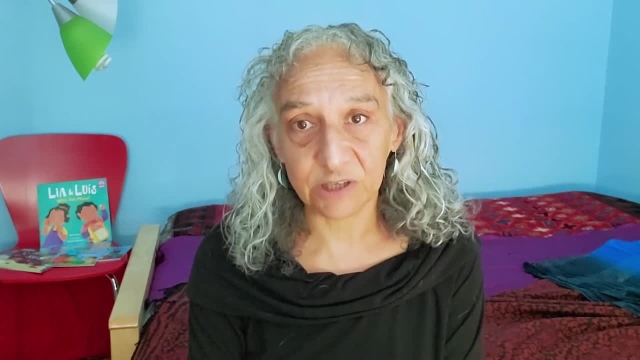 In Bracelets for Bina's Brothers. Bina wants to make her brothers bracelets with special patterns for the Raksha Bandhan holiday, But it's harder than she thought. As Bina makes the bracelets, she explores patterns. Some researchers say that patterns are one of the most important math topics for young children.